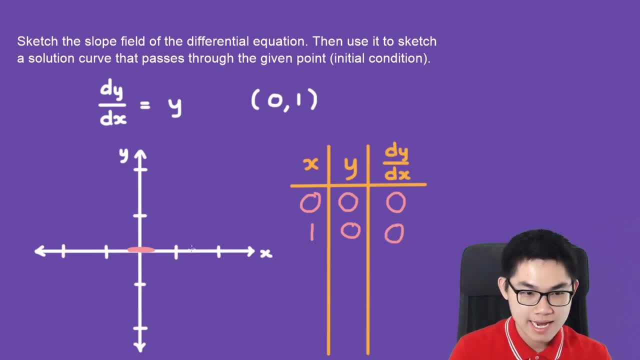 on y, so it's also going to be 0 and that's going to be a horizontal line. So maybe you notice that we don't need x as long as y is at 0.. The slope will also be 0. so on this x-axis, where y is equal to 0, all the slopes will be. 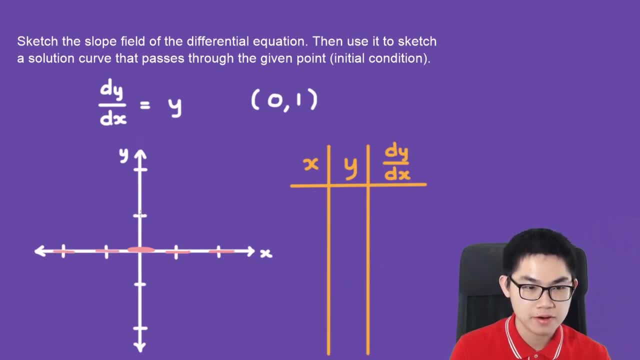 horizontal. Let's go up here What is 0 and 1?? So, 0 and 1, the slope will also be 1, and when the slope is 1, you just draw it like this: How about this point, which is 1 and 1, the slope will also be. 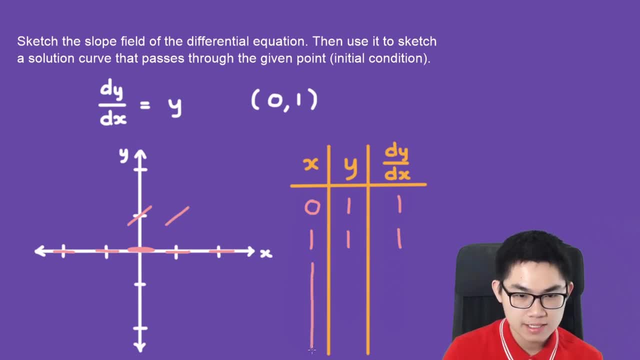 1. don't need x, and as long as y is one, the slope will be one. on this line right here, where y is equal to one, all the slopes will be ones. what happens? when y is two, the slope will also be two, and x does not matter. so when y is equal to two, which is here, the slope will be two. 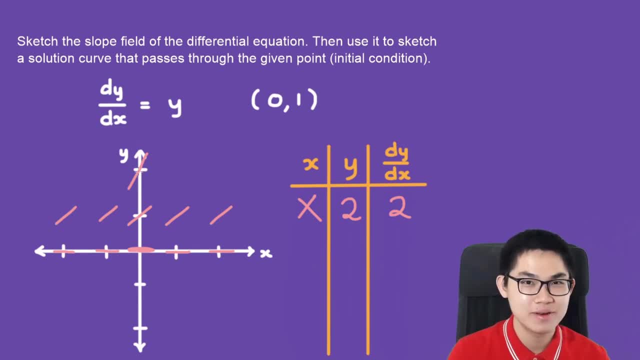 instead of one. so you just draw it slanted upwards a little bit more. how about when y is equal to negative one, which is this line? here, the slope will also be negative one. so a negative one slope would look something like this: and how about negative two? it will slant down a little bit more. 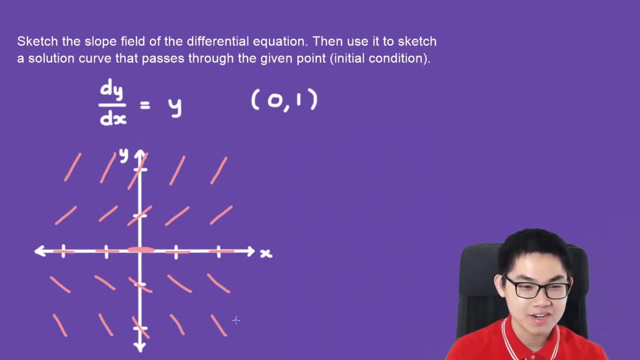 and we're almost done. so what we have here is called the slope field, or also known as the direction field, and we have this point, which is the initial condition, and that's at zero one. so let's draw the solution graph: here the slope is one, so we just kind of draw like this: and here the slope is zero. so i'm guessing. 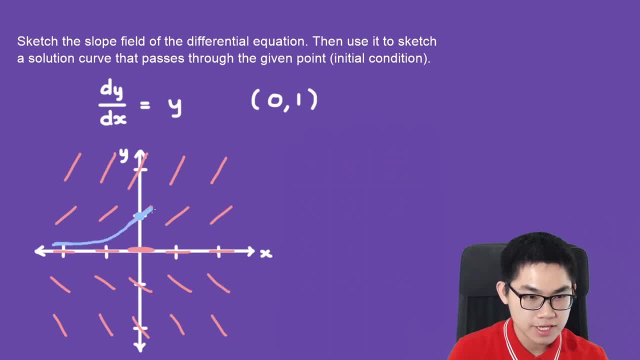 it's like here, and then it starts increasing and then it reaches here, and then here the slope is bigger, so we have to slant it upwards. so that's it. here we have the solution curve, and that solves the problem. let's do another problem this time. 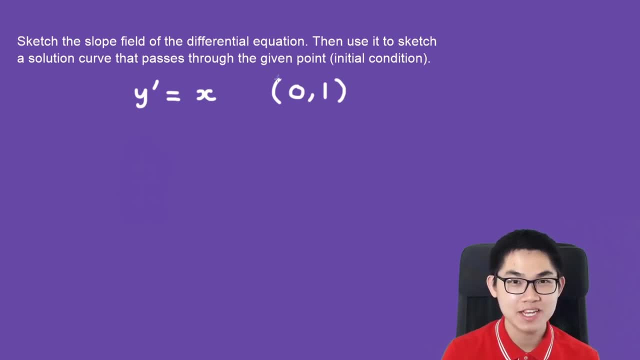 what we have to do is we have to write the slope y prime, and then we have to write the slope y prime. y prime is equal to x and we keep the initial condition the same. so here y prime is also the slope. it's the same thing as dy over the x. but instead of writing like this, i like to keep it. 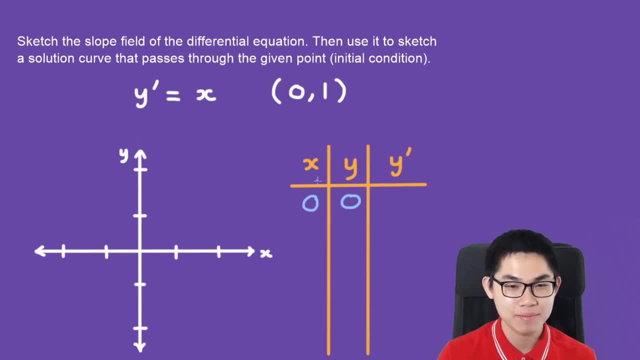 concise and just write y prime. let's start at the origin: zero and zero. well, the slope y prime, only horizontal line. now, how about 1 to 0? the slope will also be 1, which would look like this: so you notice, we don't need y. what happens when x is 2? at 2: 0, the slope will be 2, slant upwards a little. 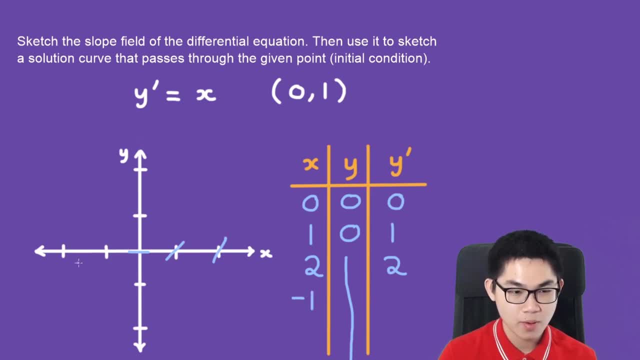 more about when x is negative 1 at the point. negative 1, 0. well, the slope is negative 1 as well, and here will be negative 2. now you might notice that on this y-axis, x is always going to be 0, right, so the slope on all of these points will all be zeros. so here is 0 1. well, x is 0, so the 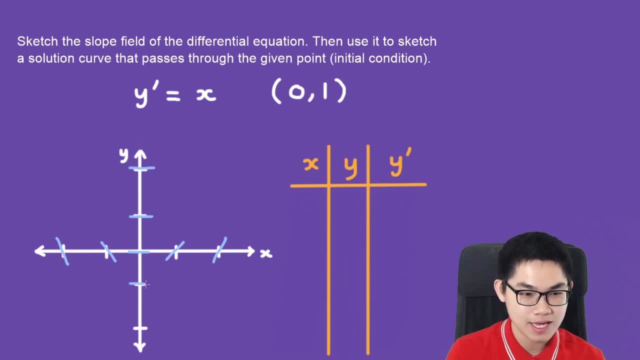 is horizontal. here x is also 0, x is also 0 and x is also 0. on this vertical line: here x is 1, you. so here the point is. so the slope is like this: here x is also one, x is also one here. same here as well. 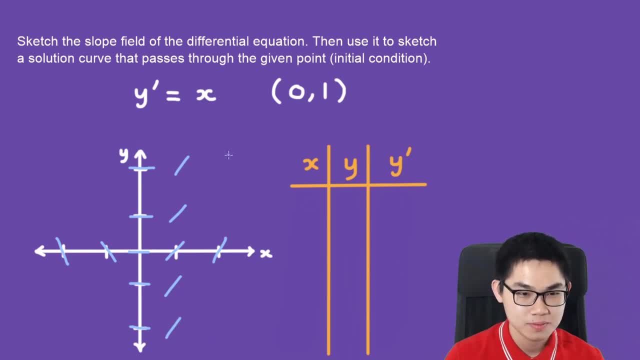 on this vertical line x is equal to two. on this vertical line x is equal to negative one. and finally, on this vertical line x is equal to negative two. last step: we put the point onto our graph and we draw the solution curve. so at this point we see that it is horizontal. so it starts out like this, and here it starts to increase and keep increasing. 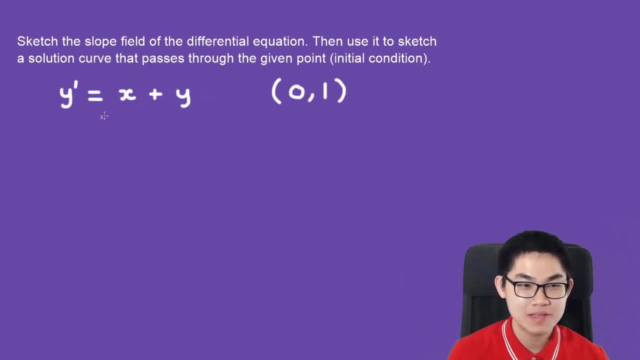 one last problem, but this time the slope depends on both x and y, so y prime is equal to x plus y, and we're going to keep the initial condition. and we're going to keep the initial condition the same. now let me show you a quick way to graph the slope field. 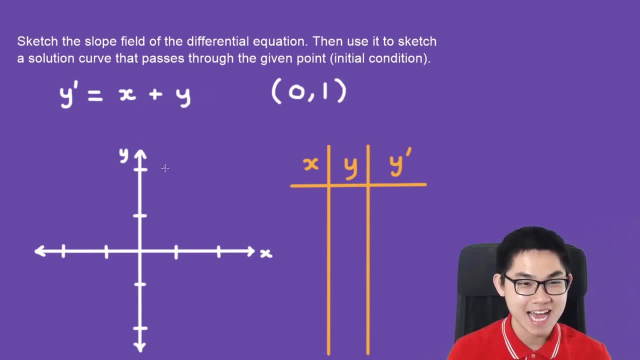 so when you see x plus y, you can see that if x is, let's say, negative two and y is positive two, then x plus y will give you zero right, and if it's negative one and one, the slope will also be zero. and if this is zero, this is also zero.